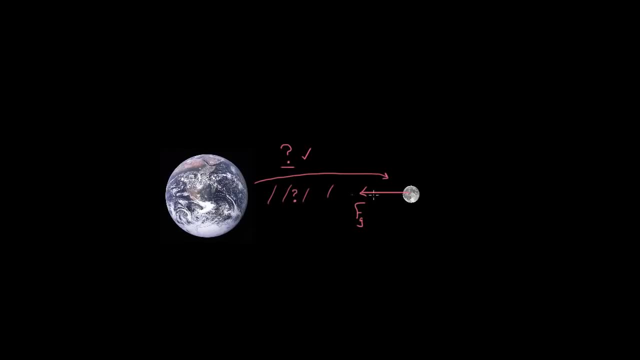 Is there something in between here that's actually letting the Earth pull on the Moon? And so, finally, when people were dealing with this electrical force, the phenomenon, they decided: all right, it's time. It's time to answer. how do two objects exert forces on each other across what are potentially vast distances of space? 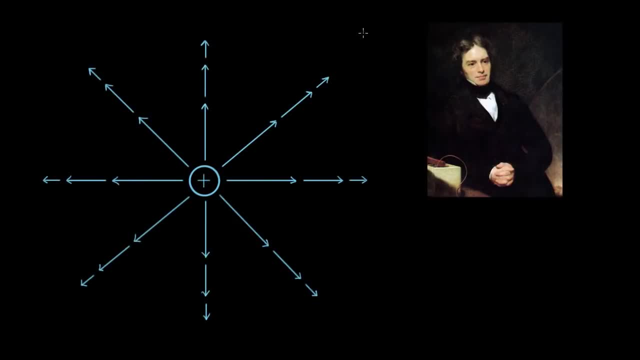 And the person who came up with an explanation was named Michael Faraday. So this is Michael Faraday, right here. He did his science in the 1800s, generally regarded as one of the most important physicists- slash chemists- of all time, really. 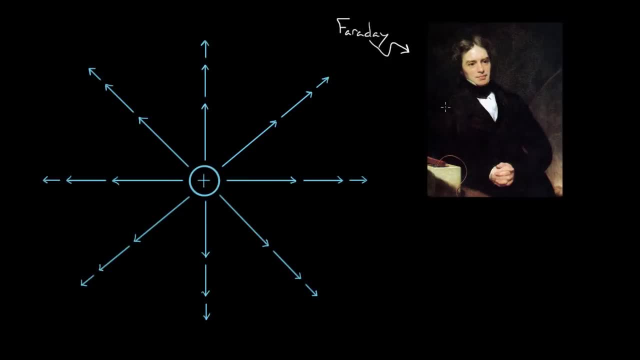 And what Faraday said is this. He said, guys, here's how it's working, So this positive charge over here. So forget about it. Forget about the other positive, Forget about this green positive for a minute. Let's just focus on this blue one. 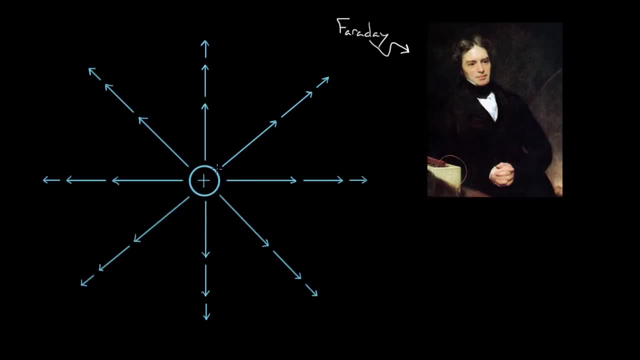 He said: here's what the blue charge is really doing. He said: this blue charge is creating an electric field all around it And we'll abbreviate this electric field with a capital E And since it's a vector, we'll put a little vector arrow over the top. 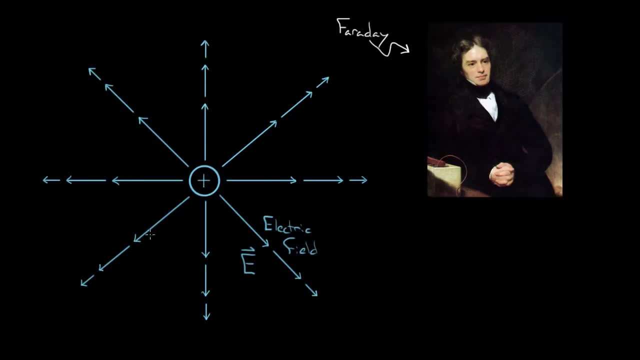 So Faraday said, this positive charge creates an electric field everywhere around it at all times, whether there's other charges nearby or not, And the electric field gets weaker and weaker the further out you go. So near the charge you've got a big electric field. 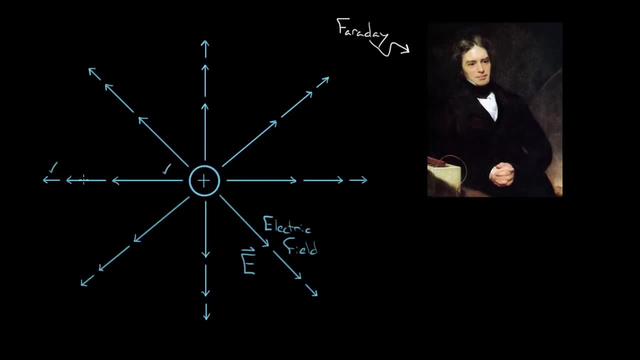 And then the further away you go, the weaker the electric field is. So this is kind of like a spider web surrounding a spider, except the spider is like the charge and the web is like the electric field. Now you've got to be careful. 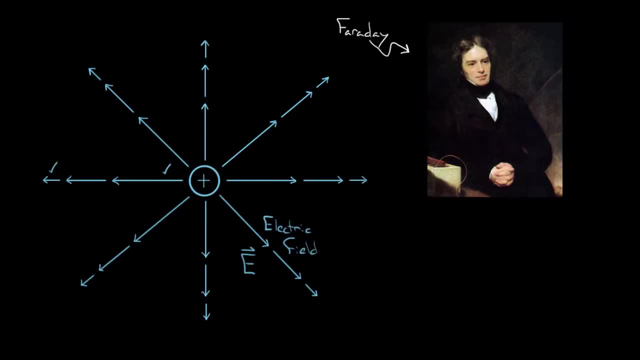 People see this and they think, oh, this is just like electric force, right, But this is not a force. These vectors here are not forces. This is where people get really mixed up. They look like forces because people are like we used arrows to draw forces before. 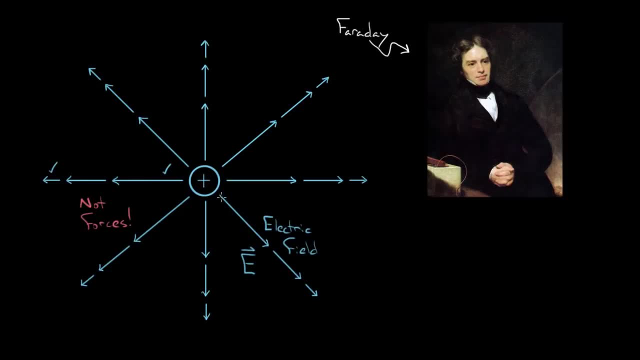 Aren't these just forces? They're not. It's a vector, So we represent them with arrows. But the electric field is not the exact same thing as electric force, So you've got to keep that straight. They are not the same thing. 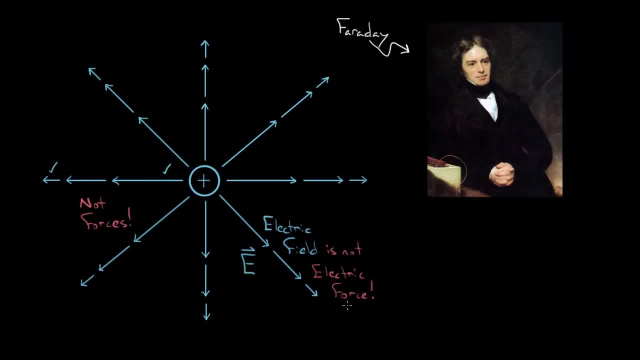 They're very related but they are not the same thing. Electric force is F, We represent it with F and maybe a little E for electric force And since it's a vector, we could draw it with a vector sign. But the electric force is not the same thing as the electric field. E. 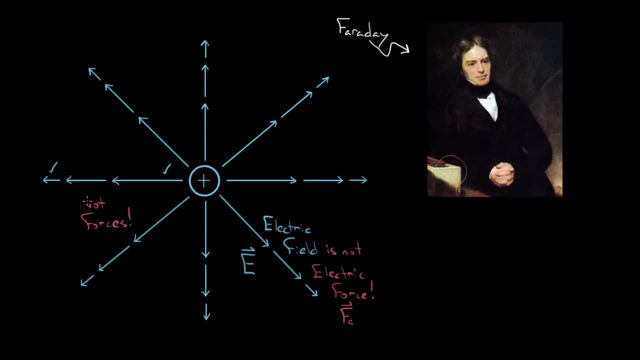 How are they related? Here's how it works. So, even though the electric field is a vector, we can draw it with a vector sign. So if this is not a force, it can cause an electric force on other charges. So, as it stands right now, if all we had was a positive charge creating its electric field in the region surrounding it, 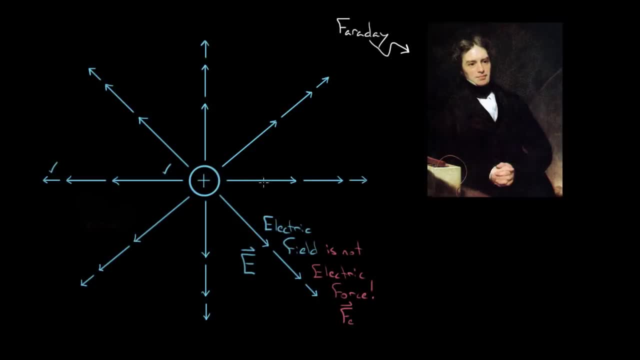 there would be no electric force. You need two charges to have an electrical force. This charge is not going to exert a force on itself, So this blue charge. and to keep these all straight, let's just give this a name. We'll call this Q1.. 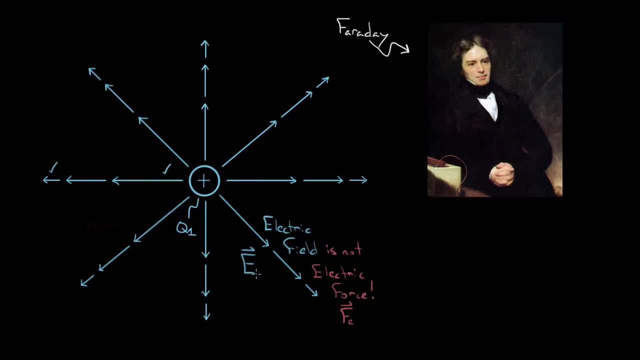 This charge, Q1, creates an electric field, but that electric field I'll call it E1, because it's created by Q1. This E1 does not exert a force on Q1. It will exert a force on any other charges that wander into this region. 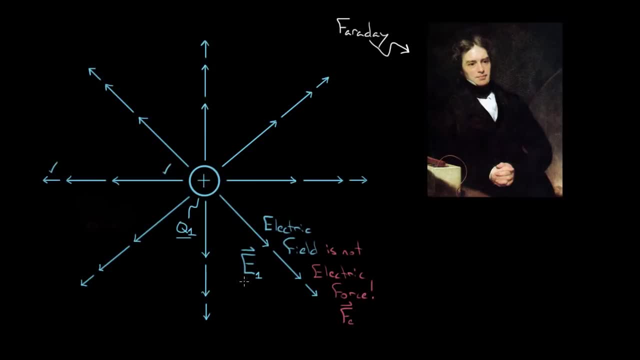 So this electric field that gets created by Q1 just sits and waits patiently, just like a spider web waits around the spider for another charge to wander in and then it'll exert a force on it. So let's put another charge in here. 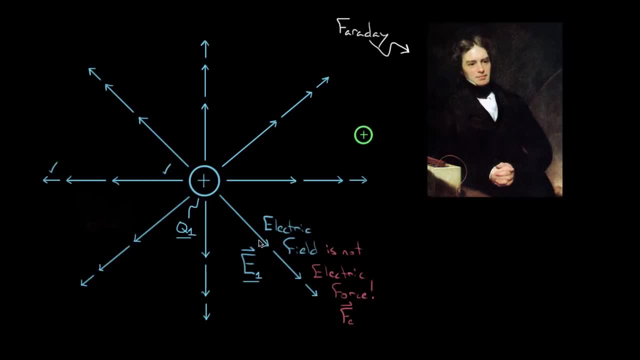 Let's say, this positive charge wandered into this zone for some reason, Who knows why. If it wanders into this region, there will be a force on it. There will be an electric force on this charge. And here's the story that Michael Faraday told us. that made us feel better. 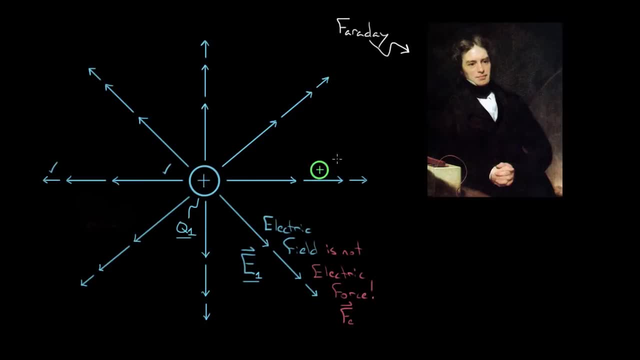 about how this force at a distance works. Michael Faraday said: here's what's really happening. This positive charge Q1, is creating an electric field all around it, including this point over here where Q2 is, So we'll call this charge Q2.. 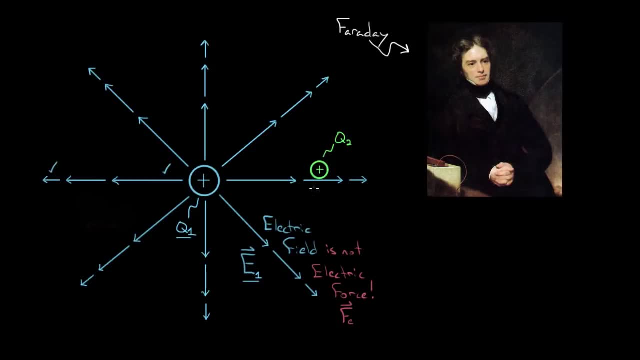 So there was already an electric field at that point that was being created by Q1. And now, when this Q2 wanders into this region, the Q2 just has to look at its immediate surroundings. this point, right here It sees this electric field. 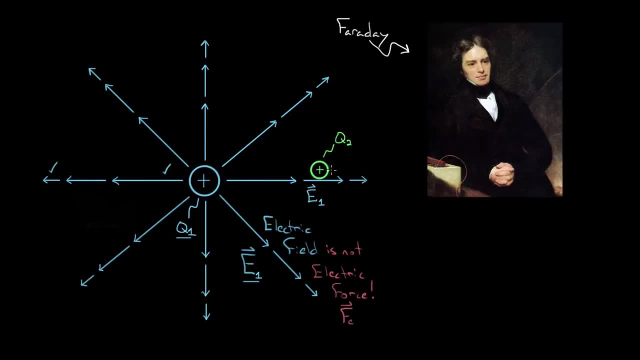 It senses it And it knows. OK, an electric field pointing to the right, that's going to cause a force on me, to the right, So it causes an electric force. The electric field is not an electric force, but it will cause an electric force on a charge that wanders around into it. 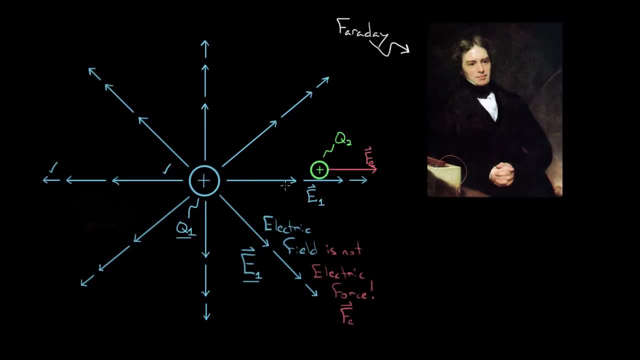 And you might wonder how is this any better? Well, it keeps things local, So physicists like it when things stay what we call local- And by local we mean OK, this charge Q2, in order to figure out what it should do. 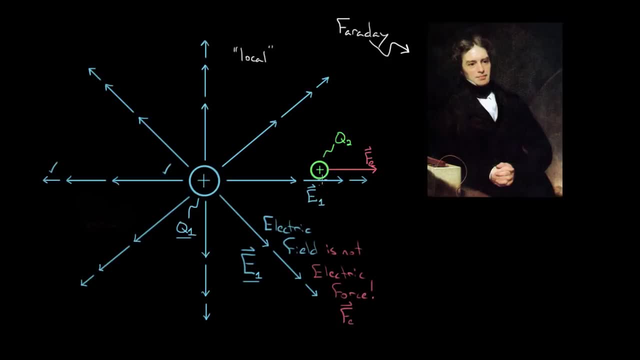 all it has to know about is the things in the space immediately surrounding it. So it just samples the electric field. at this point, right here, It says, oh, there's an electric field pointing this way. I'm going to feel an electric force in that direction. 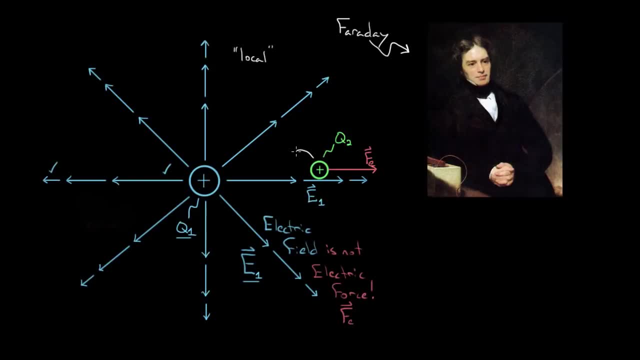 In other words, it doesn't have to know, It doesn't have to say: oh, there's this positive charge on this other side of the galaxy And that's the thing exerting a force on me. Nope, It just knows. oh, there's an electric field right here. 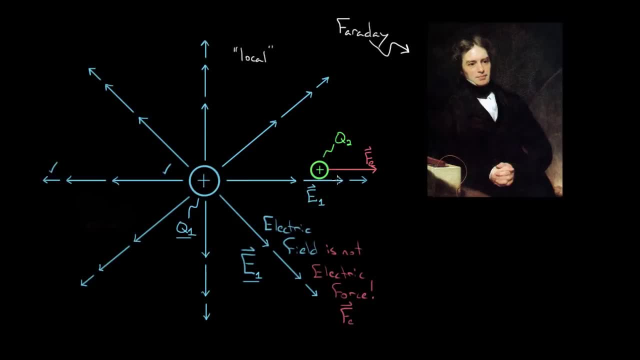 That's all I need to know to figure out the electric force on me. So that's sort of how Faraday got around this question of how does one object exert a force on another object when there's nothing in between. He said there's a mediator, basically that this first charge creates a field everywhere. 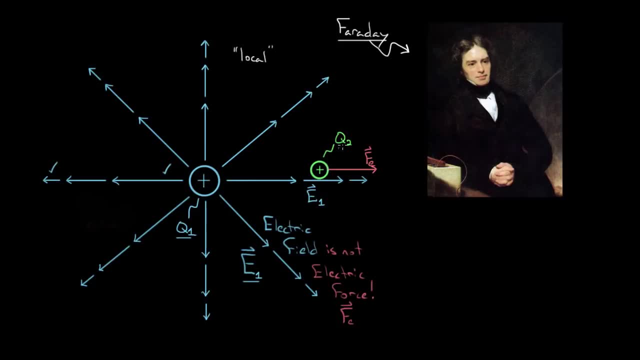 including at this point, And then that field is creating a force on this charge that wanders into that zone. So I guess, conceptually, the way you could think about it is this: This charge Q1 is creating the electric field E1.. 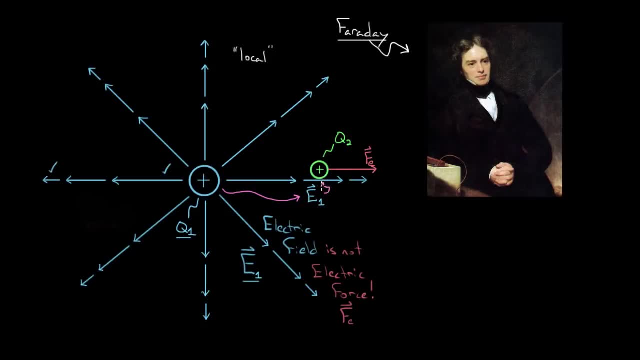 And this electric field in this region is causing a force on this charge Q2.. And that's how Q2 knows to field The force it's supposed to feel, Which keeps things local. This Q2 just has to know about the field right in its vicinity. 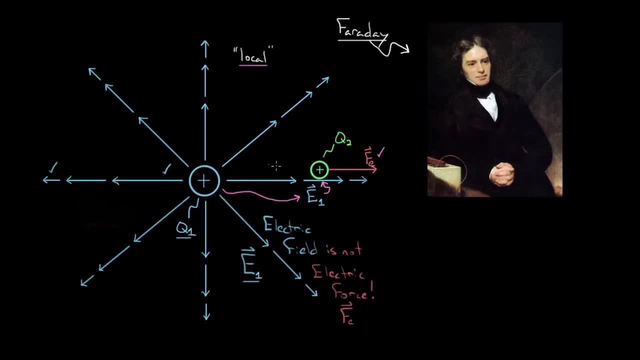 In order to figure out what to do. it doesn't have to know about things on the other side of the universe, But you could complain at this point. You might be like, wait a minute, Doesn't Q2 also create its own electric field? 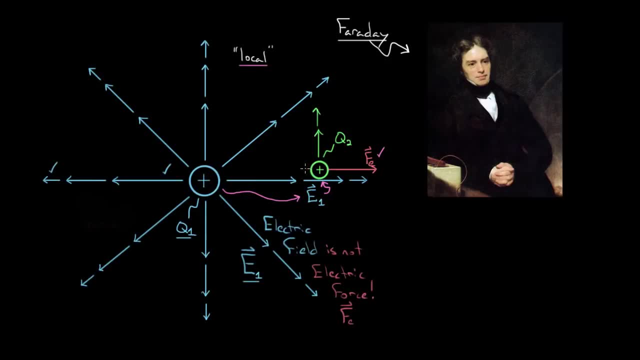 Wouldn't Q2 also create an electric field everywhere around it? We could call that E2,, since it's created by charge 2.. Doesn't it create its own electric field, just like all charges do? Yeah, it does. In fact, it'll create an electric field over here. 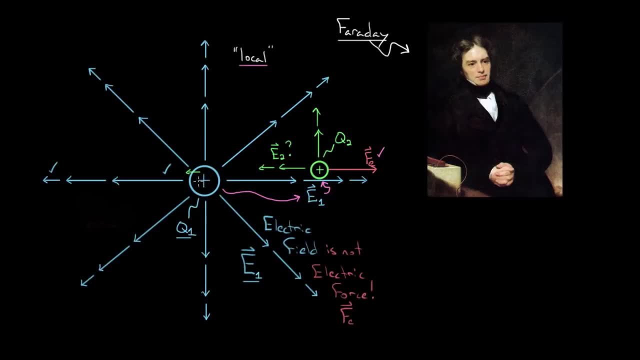 Next to Q1. And that's how Q1 knows that it's supposed to feel the force it feels in the direction that it feels it. So that's how these charges talk to each other. You could think about it that way. The way charges talk to each other is with the electric field. 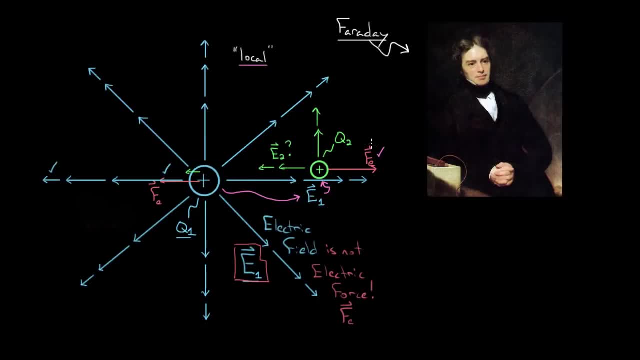 One charge creates an electric field over by the other charge, That charge feels a force. The other charge creates a field by the first charge. That first charge feels a force. So conceptually, that's how this electric field works And that's what it does. 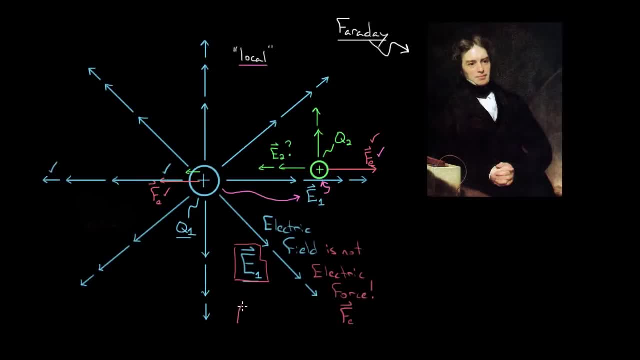 So at this point you might not be impressed. You might be like: are we just making up a story to make ourselves feel better here? Is it just some elaborate fairy tale that makes it so that we don't feel so awkward talking about things exerting forces on each other at a distance? 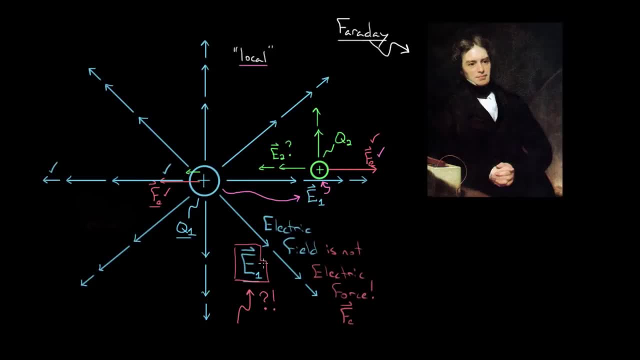 Is there any benefit for doing this? And there is. There's a big benefit, Mathematically, in terms of physics. talking about the electric field makes describing the physics way easier And in fact it makes it so that you don't even have to know about the charge creating that field at all. 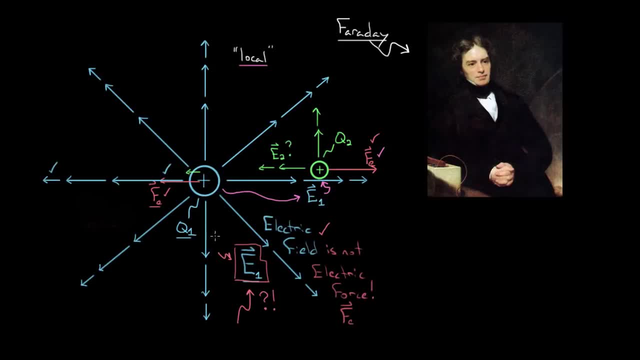 If you have a way of knowing the field, even if you don't know what charge is creating that field, you could figure out what the force is going to be on any charge in that field without even knowing the charge that created that field. And that turns out to happen a lot. 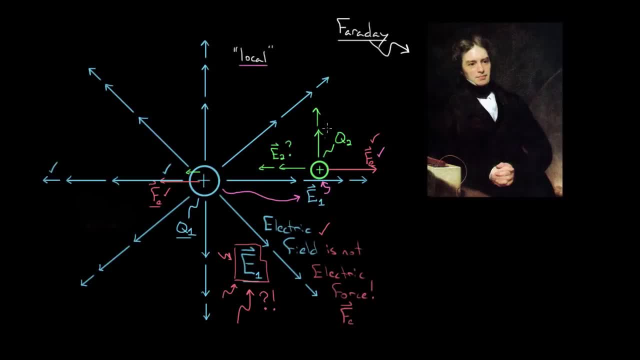 So knowing the electric field is extremely useful. It lets you determine the electric force on a charge, even if you don't know what charge is exerting that force. So up to this point I've been trying to motivate why we would want this idea of the electric field. 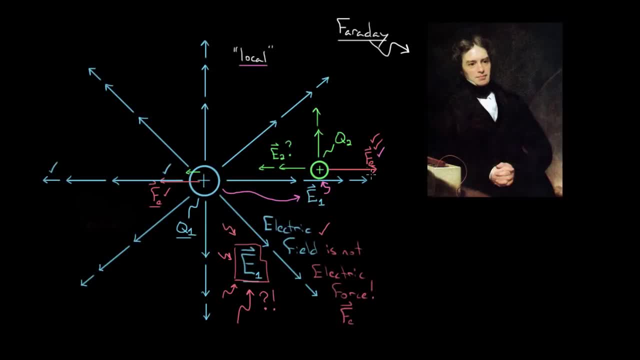 why physicists would come up with this idea. But I wouldn't blame you if at this point you weren't thinking: I still don't know what electric field is. I know what it isn't. Electric field is not electric force. But what exactly is the electric field? 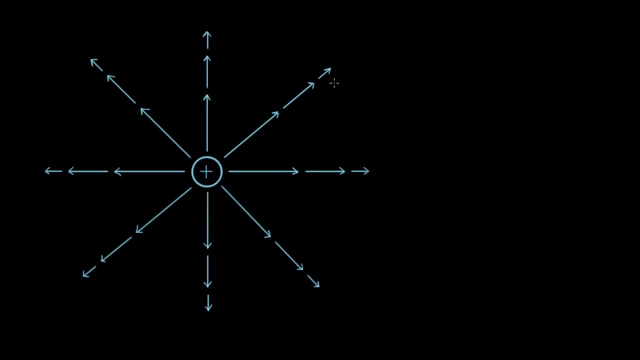 So let me give the electric field a proper definition here. The electric field E at a point in space is defined to be the amount of electric force per charge exerted at that point in space. So this is what the electric field is: It's the force per charge. 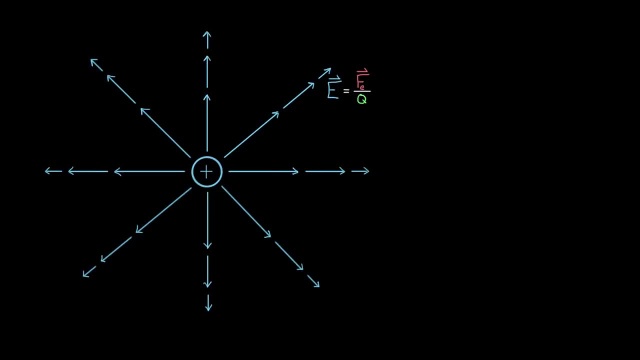 And the way physicists usually think about this is: imagine throwing a test charge in here. We call this a test charge. We like to imagine that this charge is really little, so that it doesn't completely like swamp and overwhelm the other charges, creating this field. 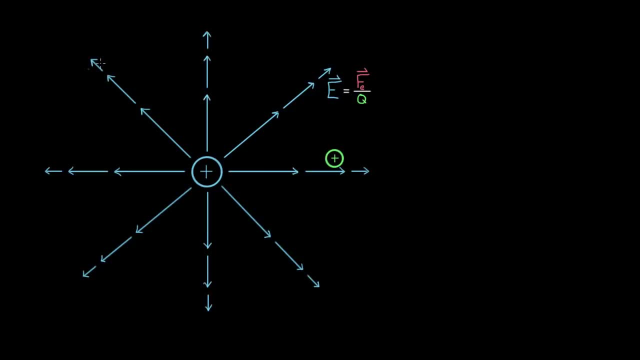 Otherwise, if you threw some huge charge in here, all the other charges would scatter and it would change the whole situation. So let's say we put a really small test charge in here If I want to know what the electric field is at a point in space. 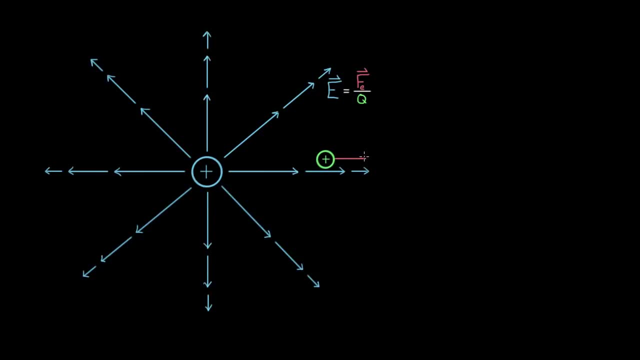 I could just bring my test charge over here, measure the amount of electric force on that test charge and then I just divide by how much charge was there on that test charge. So what was the charge of that test charge? I'll call this charge 2.. 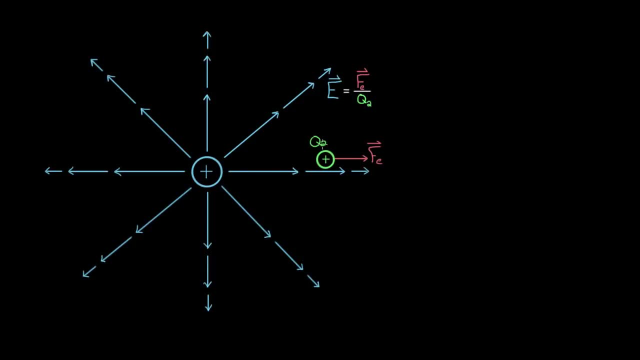 If I take the force on charge 2 divided by charge 2, that would be the value of the electric field at that point in space. So this is how we define the electric field. The definition of electric field is the amount of force per charge. 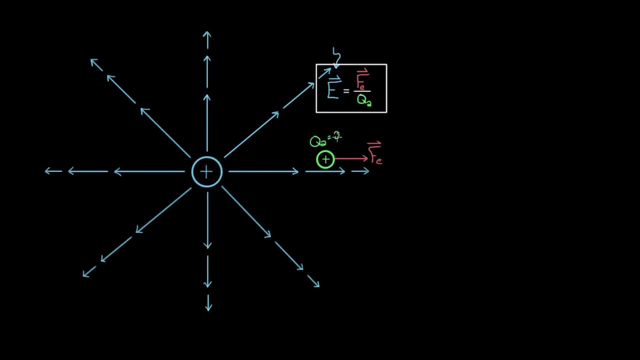 In other words, let's put some numbers in here. Let's say Q2 was 2 coulombs. This is actually an enormous amount of charge. This is kind of an unrealistic example, but it'll make the numbers come out nice. 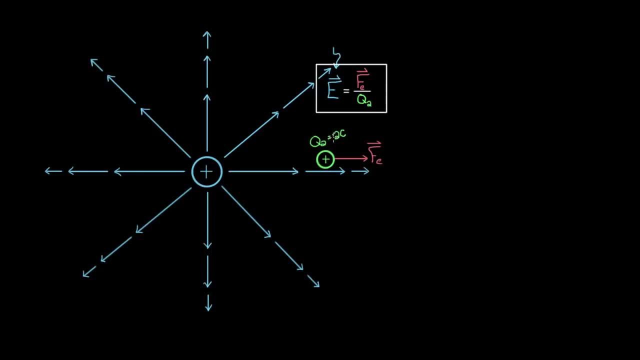 And conceptually it's the same thing. So say, positive 2 coulombs was placed here. That's the value of Q2.. And let's say, when we measure the force on Q2, we're getting 10 newtons of force. 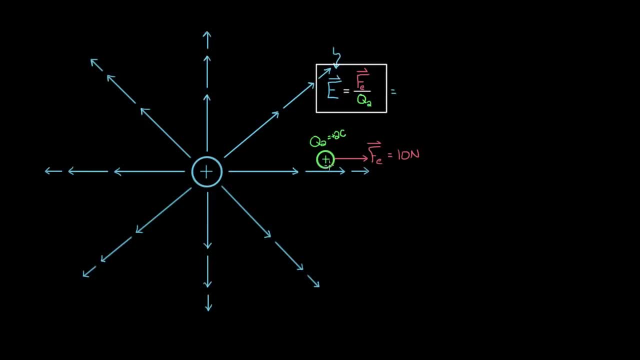 Well, in that case we could just say: all right, then the electric field in that region, at that vicinity, is going to be 10 newtons of force per 2 coulombs of charge and we get an electric field of 5,. 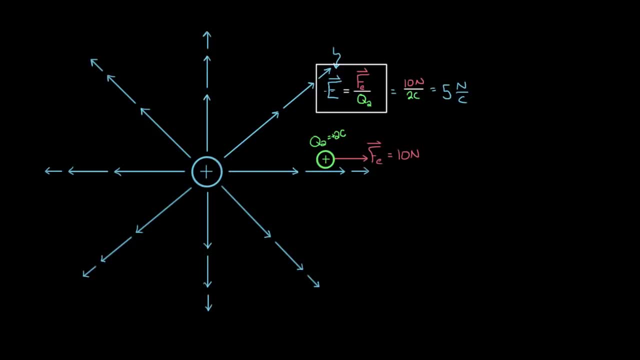 and then the units are newtons per coulomb, And that makes sense, because what the electric field is really telling you is how many newtons of force you would get per coulomb If you put more coulombs at that point in space. 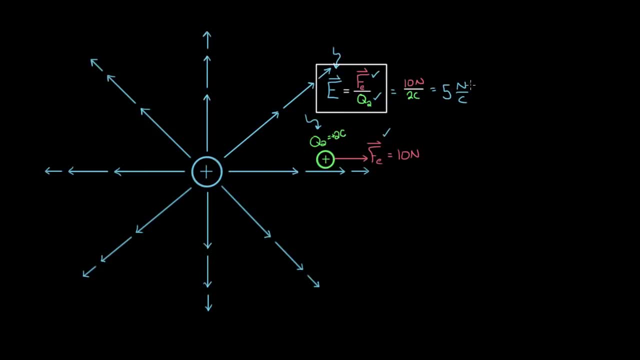 there'd be a greater force, And this number is telling you the number of newtons you would get per coulomb. So, since we had 2 coulombs at this point in space and there was 5 newtons per coulomb, 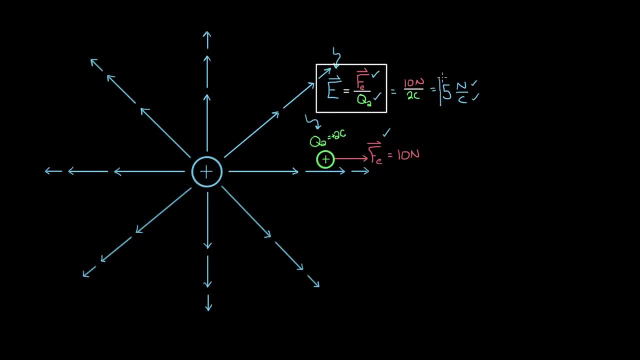 the force was 10 newtons. So this number, 5 newtons per coulomb, is important because it's the same for any charge you put there, And this is why the electric field is useful At this point in space, right here. 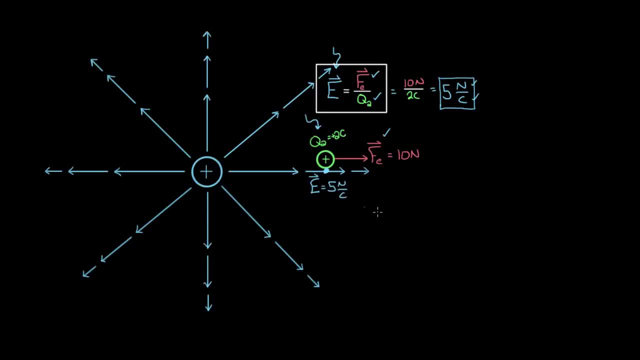 if the electric field is 5, it's 5 newtons per coulomb, no matter what charge you put there. So if I put a 4-coulomb charge at that point, since there's 5 newtons for every coulomb, 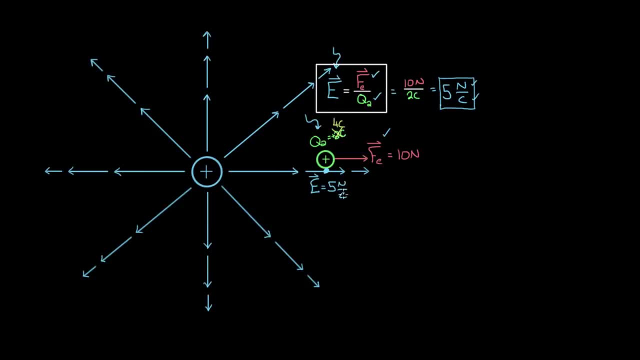 there'd be a 20-newton force there, because there's 5 newtons for every coulomb. If there's 4 coulombs, there'd be 5 times 4 newtons, which is 20 newtons. 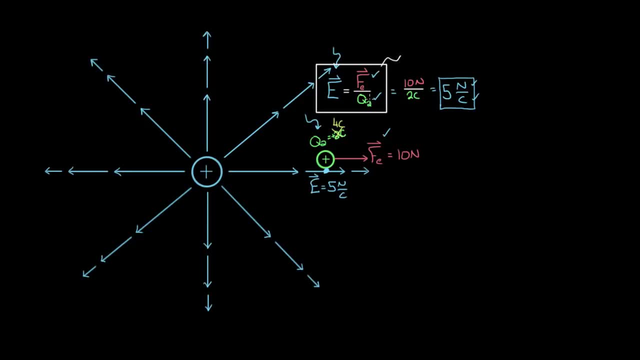 So you can imagine rearranging this formula another way. You could just multiply both sides by q and you'd get that the electric force on a charge is equal to the value of that charge at that point in space, multiplied by the value of the electric field at that point in space. 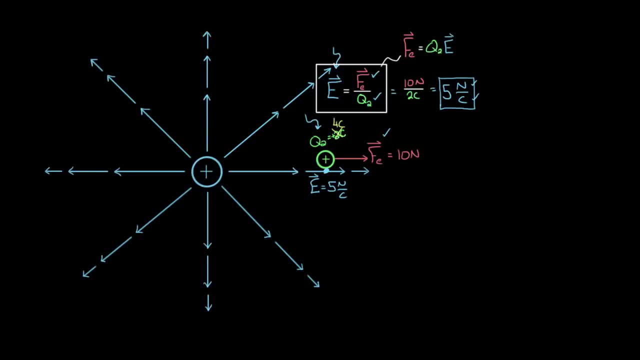 But it's important to note this electric field is not created by this charge q2.. This was created by some other charge or collection of charges. Remember this charge q1 is creating this electric field, e1, and that electric field is causing this electric force on q2.. 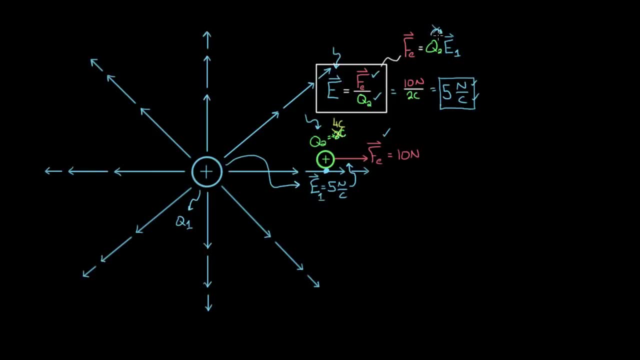 q2 did not create the electric field e1 that it interacted with. q1 created that electric field e1. So people get mixed up. They see this formula, They start to think maybe this q2 is creating this electric field. It's not.